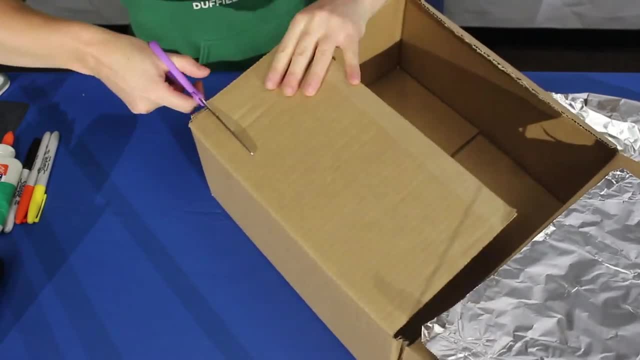 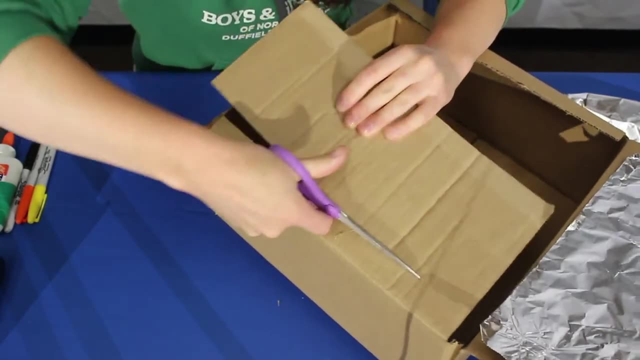 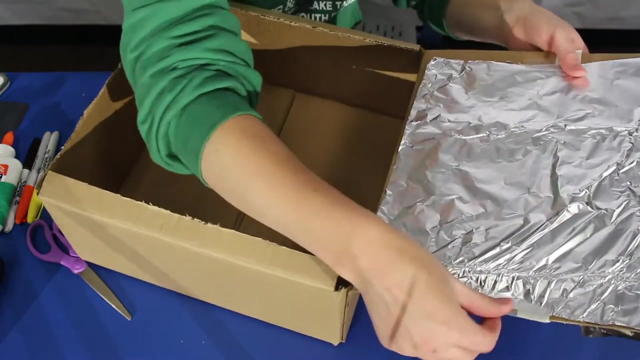 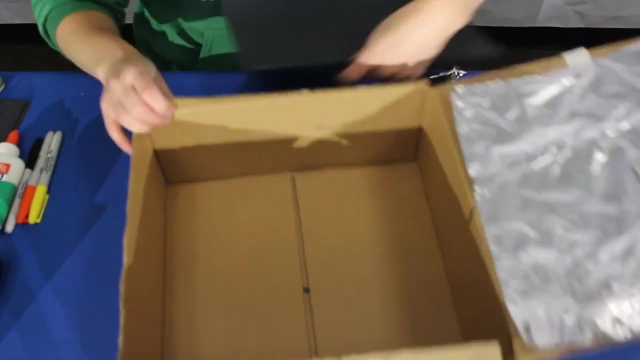 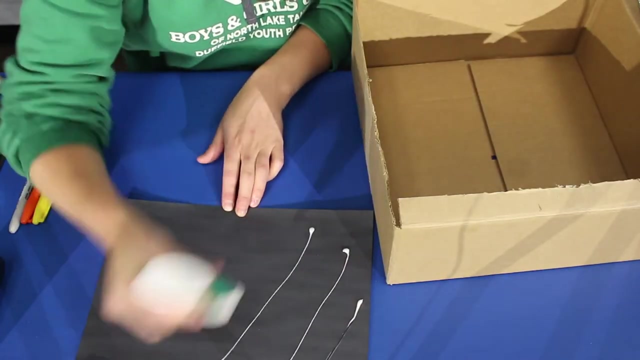 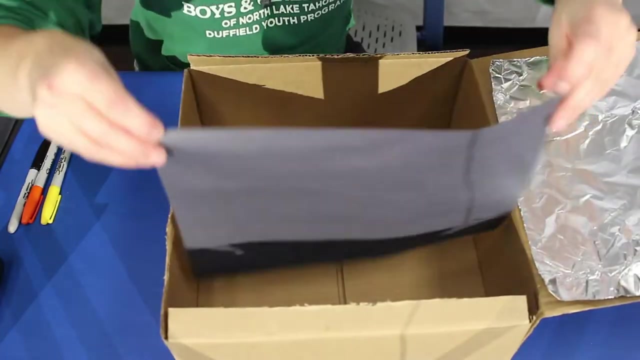 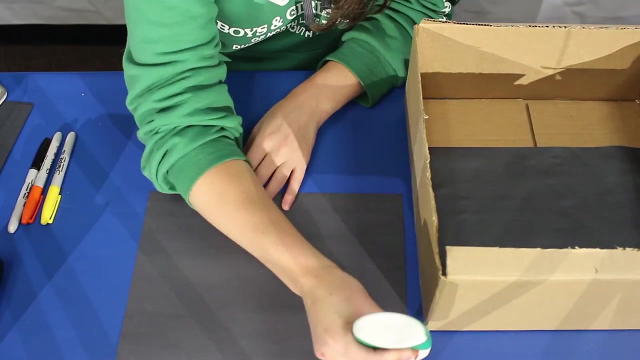 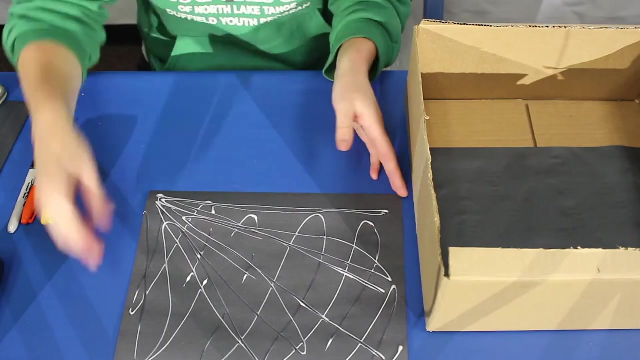 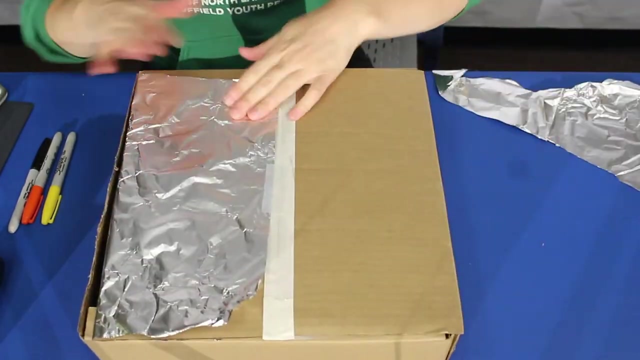 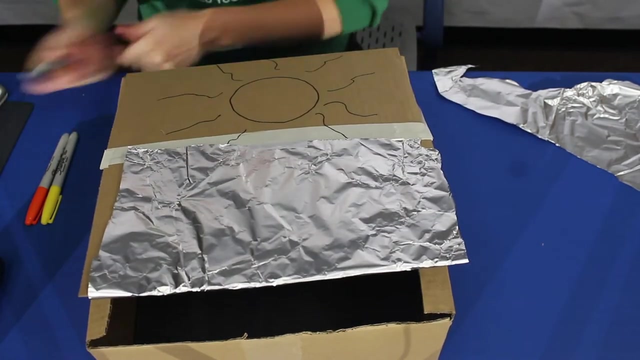 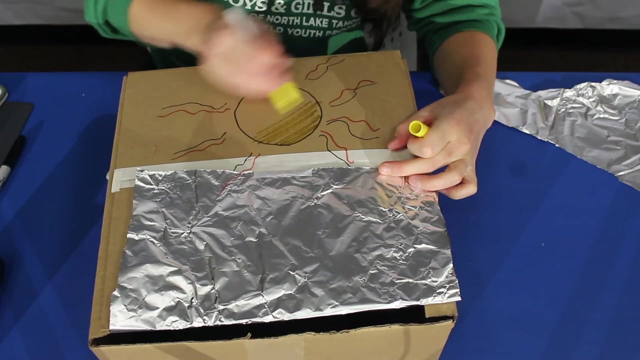 Good night, everybody. All right, the next thing that we're going to do is take some black paper and glue it to the bottom of our box or the inside of our oven. Why do you think we want to use black paper? The next thing that we're going to do is decorate. 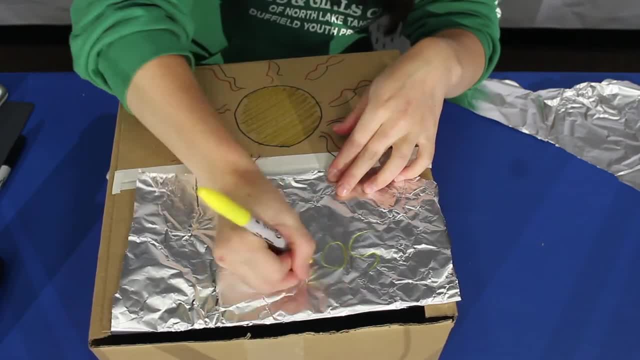 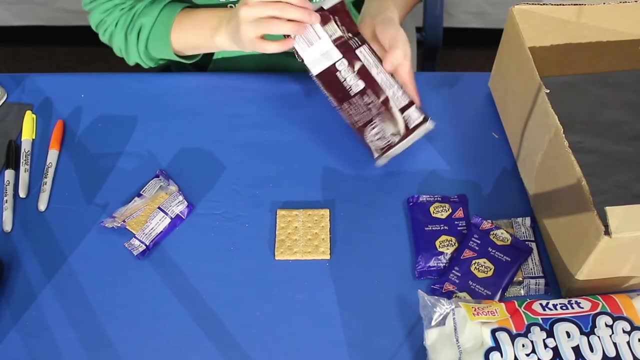 Be creative here to make your oven look however you like. All right, so our oven is almost ready. So now we need to prepare our s'mores. So we're going to take a graham cracker, put some chocolate on the bottom. 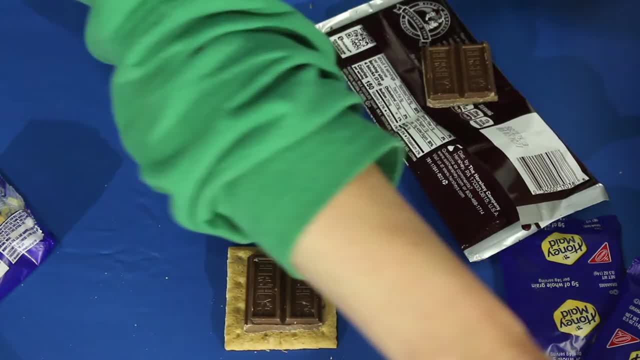 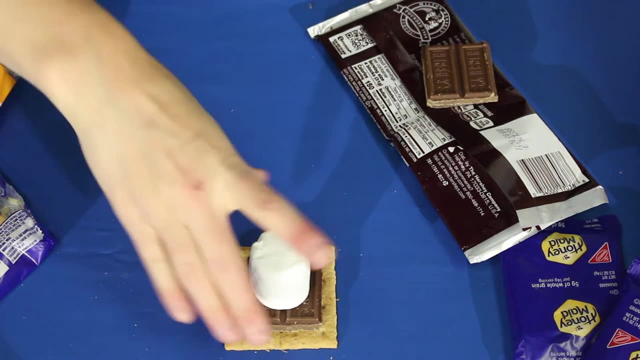 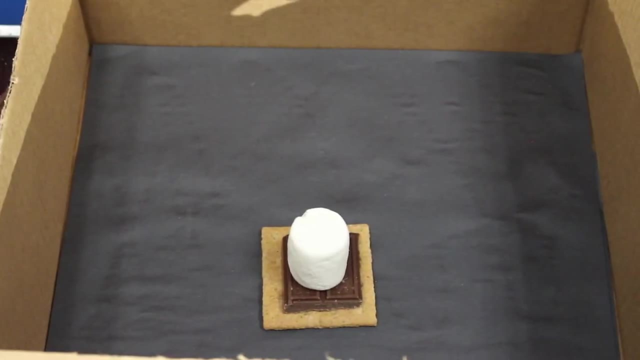 And then a marshmallow on top. You can do this however you like, but this is the way I want to do my s'more. Then we're going to place it inside our oven. You can see I have a lot more room for more than one s'more. 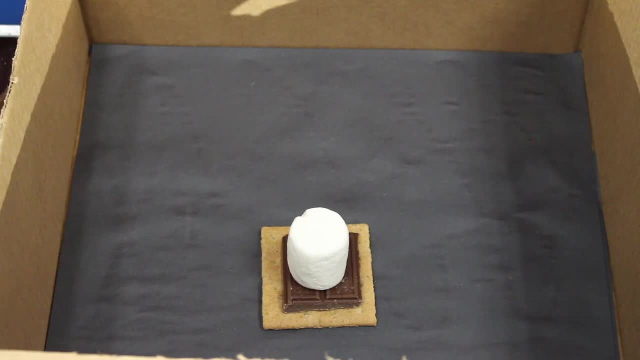 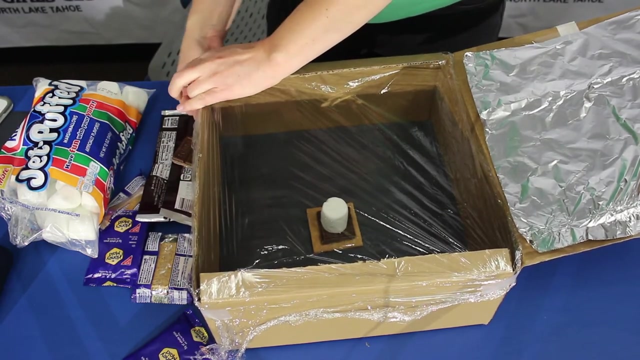 So you can make as many as you can fit, but do make sure that there's still room in between your s'mores, So don't put too too many in. All right? the final step Is to take some plastic wrap and tape it to the top of your box so that, as heat starts, 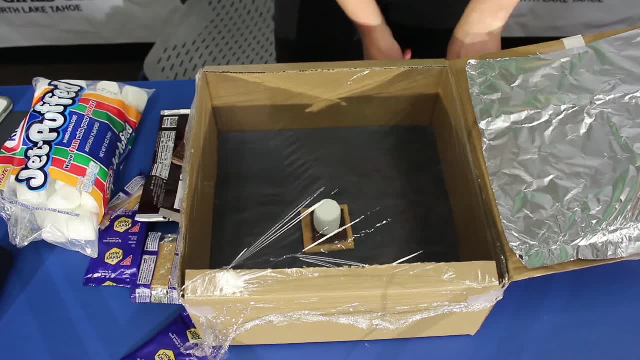 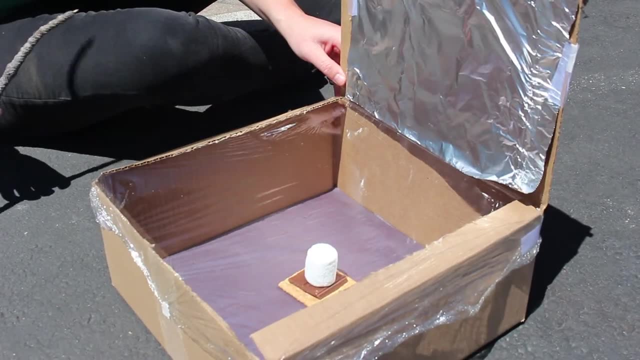 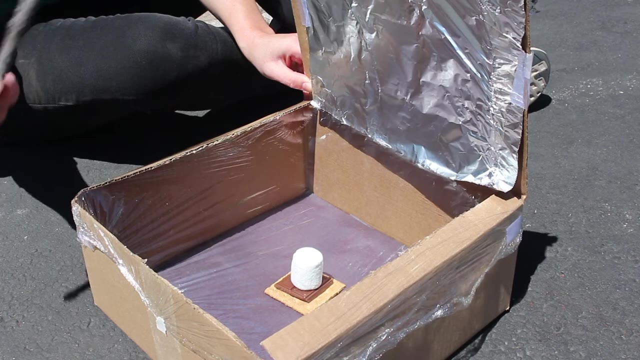 to build up inside your oven. it can stay inside your oven and won't just come out. All right, so now we get to take our oven outside and we're going to set it up in the full sun. You can do this. You can do this.